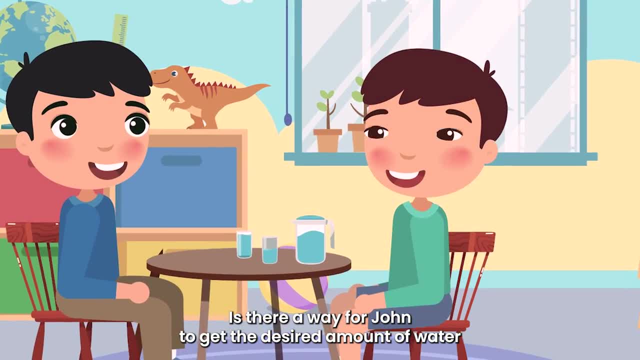 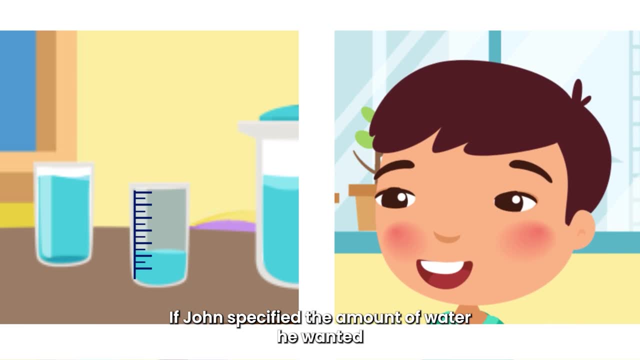 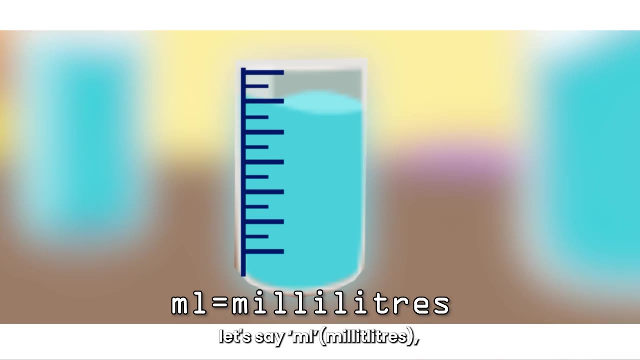 this conflict? Is there a way for John to get the desired amount of water without confusing or irritating Tom? If John specified the amount of water he wanted in a universally acceptable unit, let's say ML, Tom could understand easily. But do you think it is an achievable? 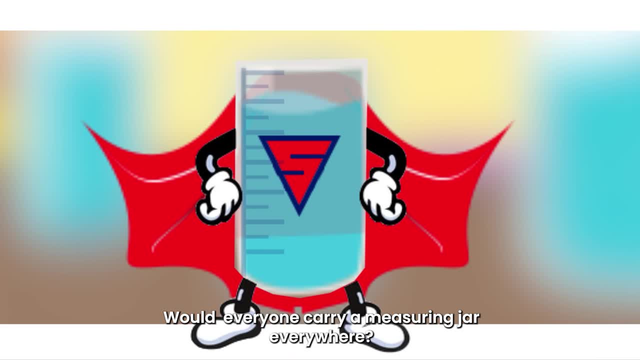 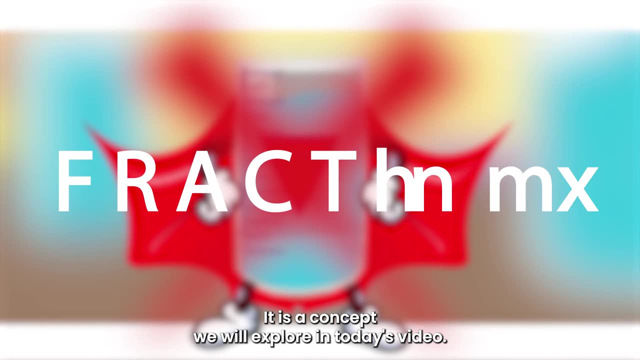 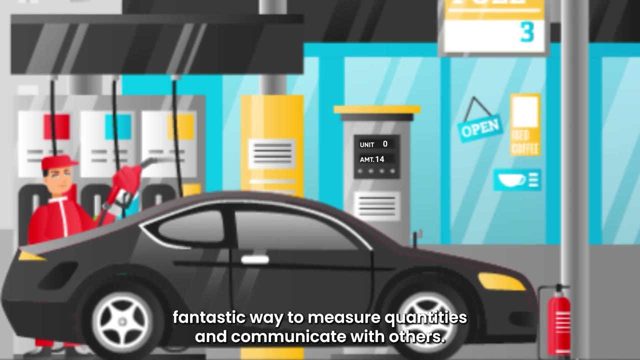 solution. Would everyone carry a measuring jar everywhere? Does not seem likely, does it? So what is the solution? It is a concept we will explore in today's video. Fractions Numbers offer us a fantastic way to measure quantities and communicate with others. If 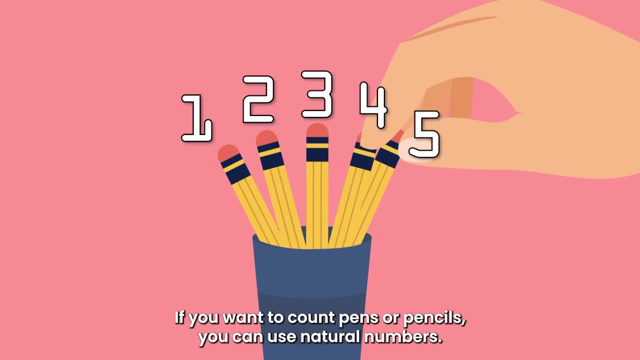 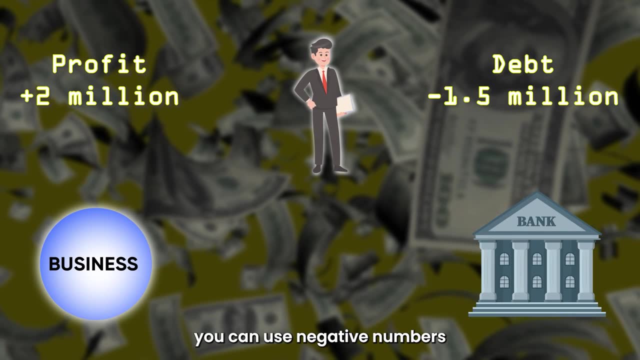 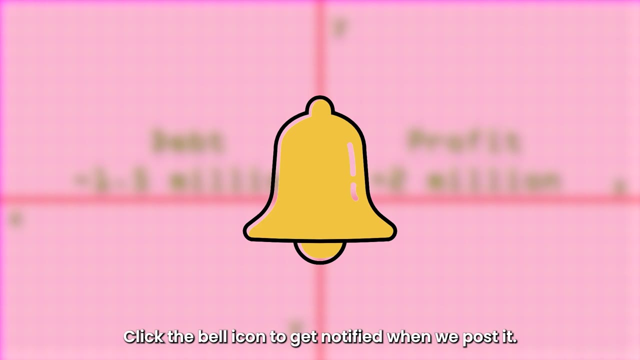 you count pens or pencils, you can use natural numbers. Similarly, if you wish to signify debt, you can use negative numbers. Confused what natural and negative numbers are? We are coming up with a video on that too. Click the bell icon to get notified when we post. 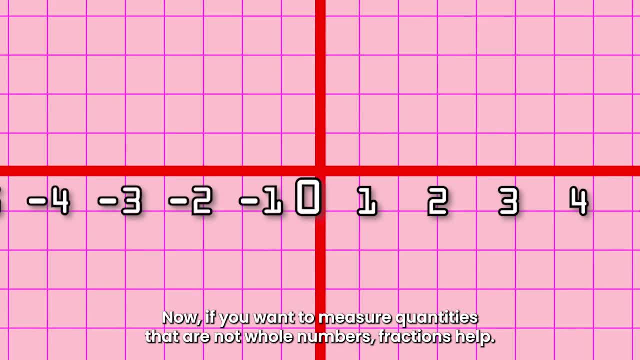 it Now. if you want to measure quantities that are not whole numbers, fractions help. Let's simplify this with an example. Here is a pizza with seven pieces. If you want to measure the number of pieces, you can measure the number of pieces If you want to measure. 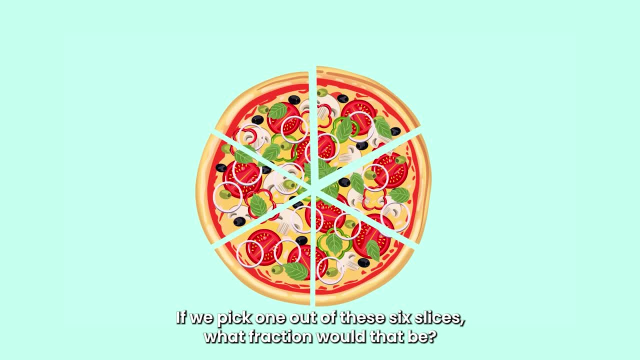 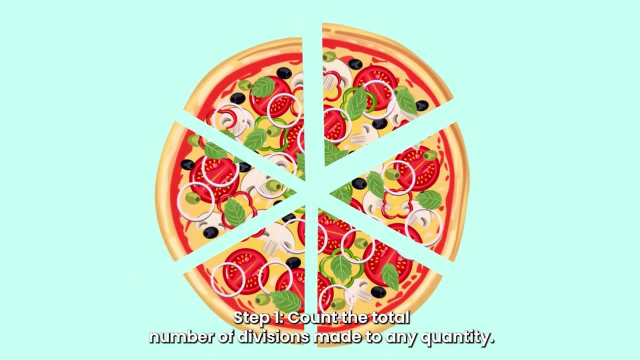 what you want to measure. you can measure the number of pieces. There are seven parts in a pizza And if you want to measure it, you can measure the number of pieces. You can do this very quickly. Here is a simple, three step way to find out. 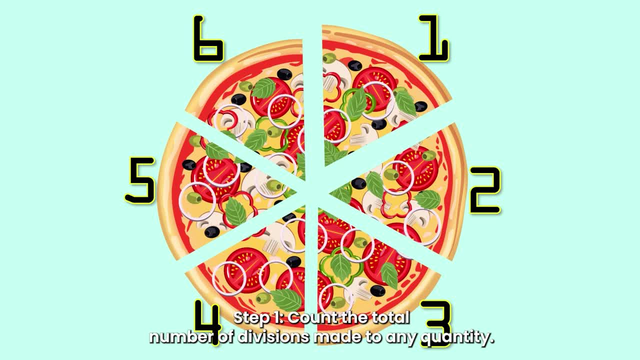 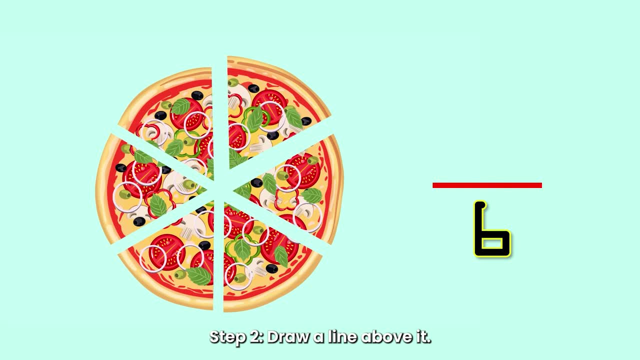 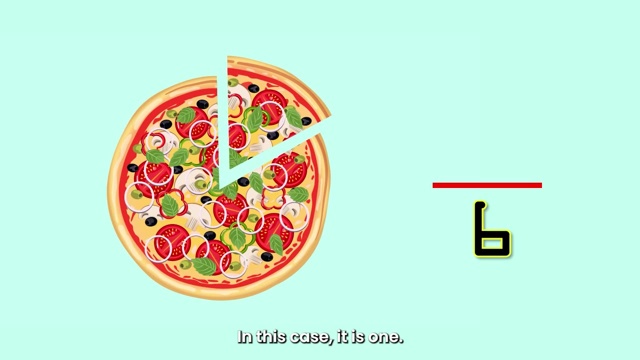 Step 1. Count the total number of divisions made to any quantity. In this case it is six. Write it down. Step 2. Draw a line above it. Step 3. Count the number of parts you are taking out of the total number of divisions. In this case it is one. Write that down, Step 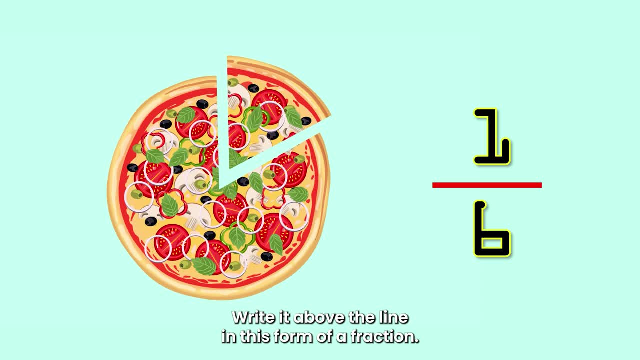 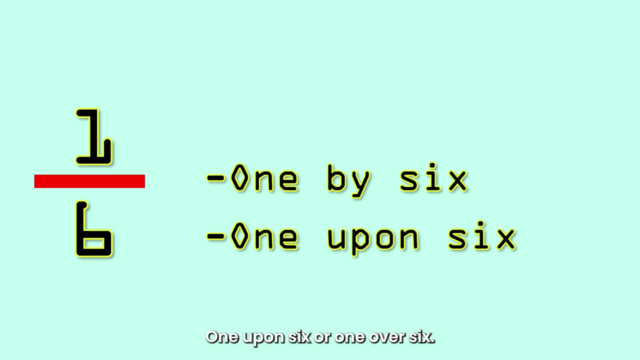 is: 1.. Write it above the line. In this form of a fraction, this slice represents 1 by 6. It is called 1 by 6, 1 upon 6 or 1 over 6.. Let's stick to 1 by 6 for now, Here. 1.